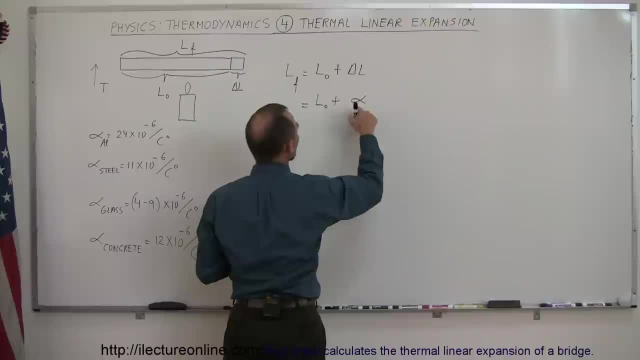 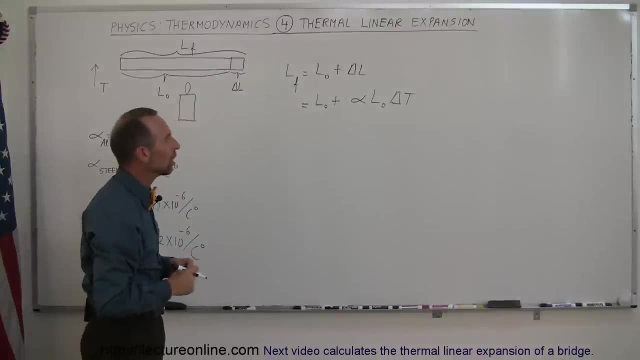 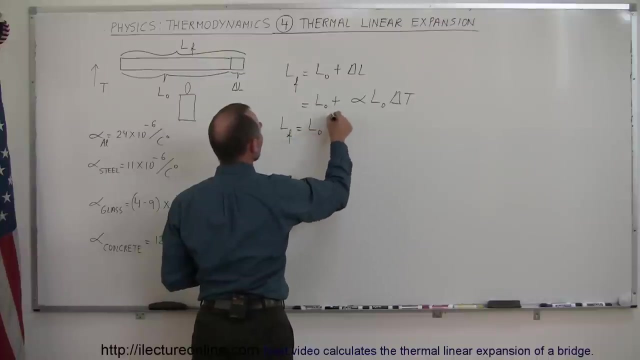 equal to the initial length plus the coefficient of linear expansion times the initial length, times the change in the temperature. So all three are factors in how much the length will change. Now notice we can factor on L sub naught. so we can say that the final length is equal to the initial length. 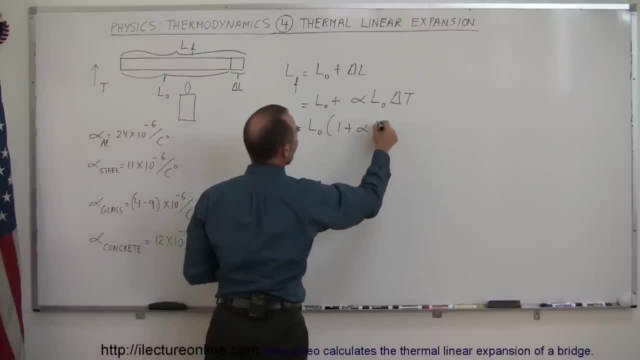 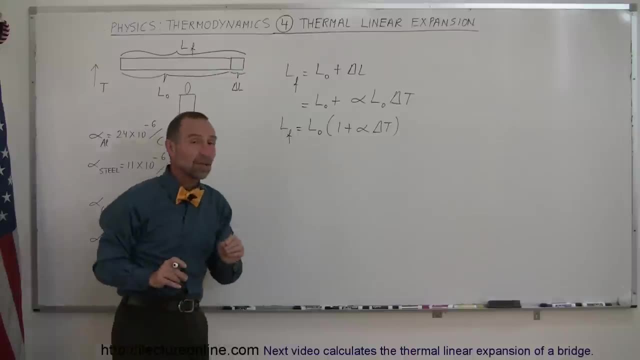 times one, plus L, Alpha times delta t. Now we're going to simplify this here, because the linear, the coefficient of linear expansion isn't in itself as linear. It changes over temperature as well. but for now, just keep things simple, We'll just assume that this is a constant. So for example, let's say we have an. 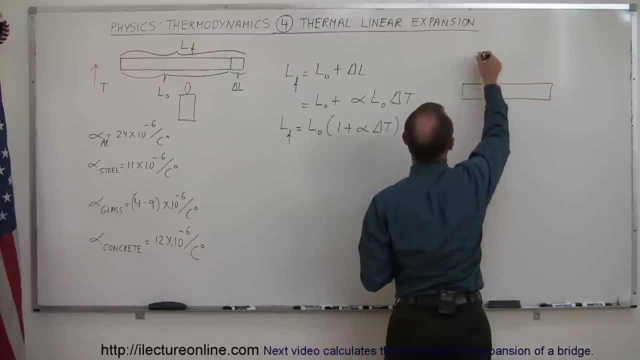 object like this that's made out of steel. So we have a steel object and let's say that the initial length is equal to 2.4 meters. Let's say the temperature initial is equal to 20 degrees centigrade and temperature final is equal to 120 degrees. 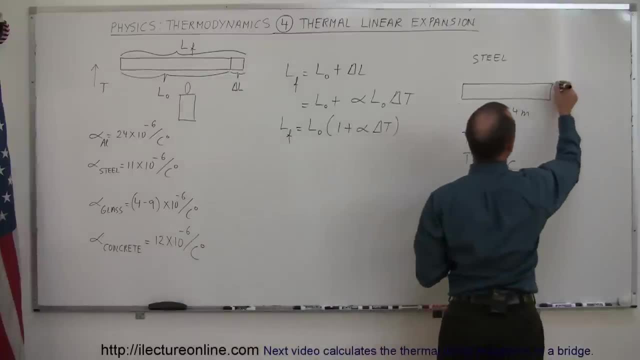 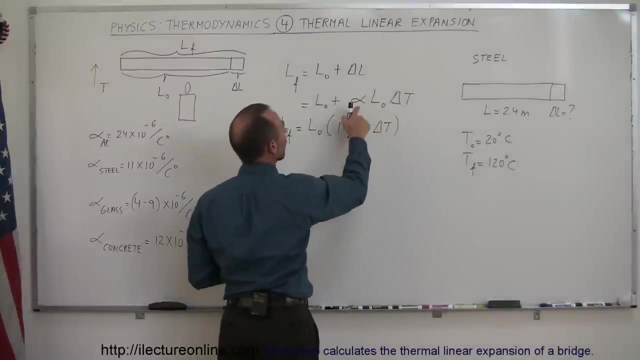 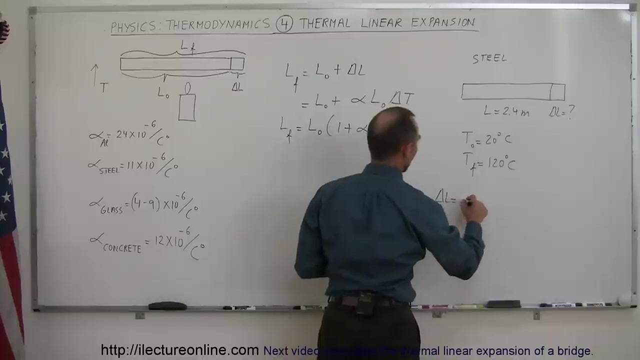 centigrade. How much longer will this object be? What will be the increase in length? What is the delta L equal to? question mark? Well, here we can see that the delta L is simply equal to the coefficient times, initial length times, the delta t. So the delta length delta L is equal to the 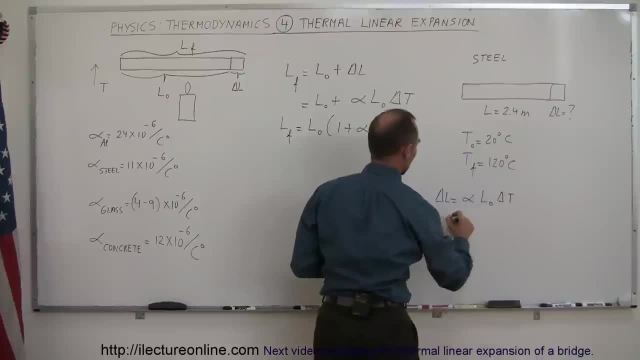 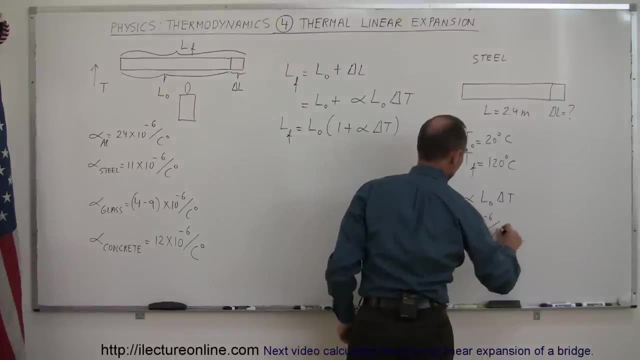 coefficient times, initial length times the change in the temperature. So the coefficient right here for steel is 11 times 10 to the minus 6 per centigrade degree. The initial length we said was 2.4 meters and the change in the temperature was 100 centigrade degrees. Notice that the centigrade degrees 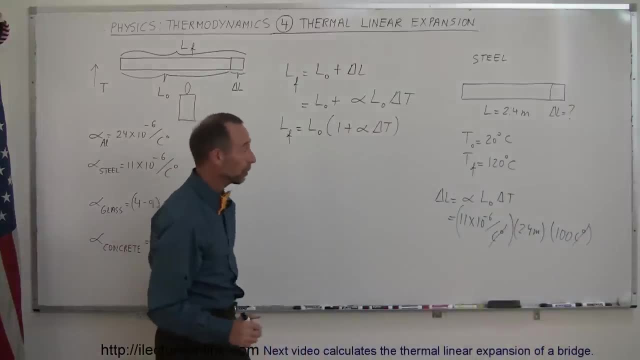 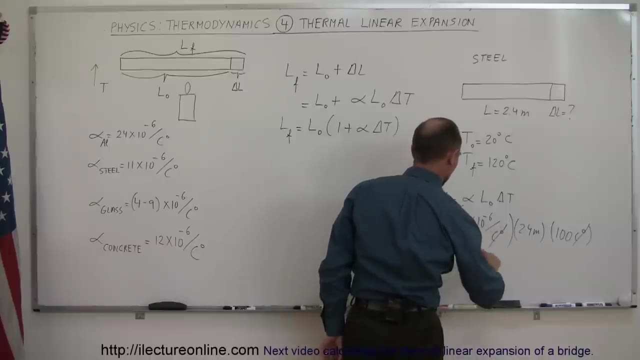 here cancels out with the centigrade degrees there, and all we have to do is multiply those together. Now, 2.4 times 11, that would be equal to. that's a 2, a 4, and a 6 here. That would be. 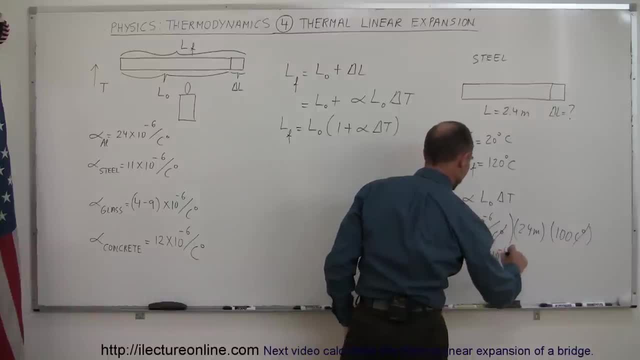 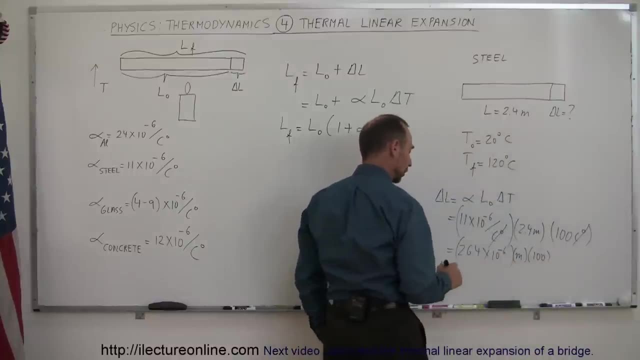 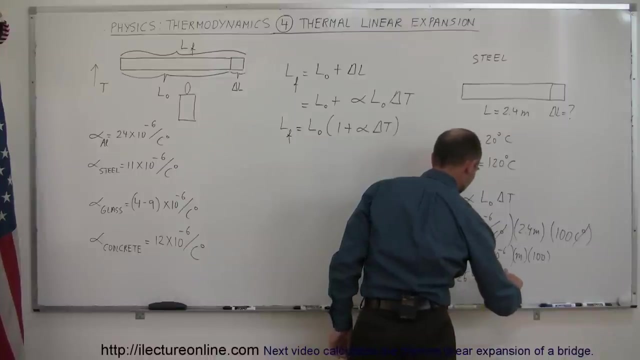 6.4 times 10 to the minus 6, and that would be meters and times 100.. Of course, 100 will take off a couple notches of the exponent there. so it would be 2, 6.4 times 10 to the minus 4 meters.